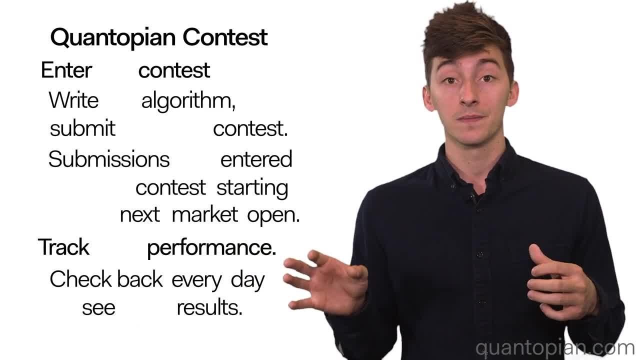 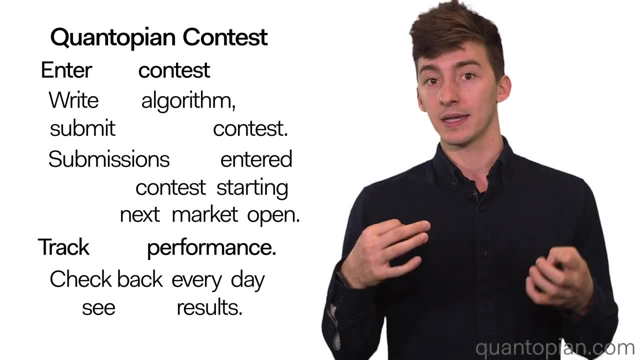 This is stuff like the an, uh. We can cut all of these out without losing the information density, density of our corpus. So we filter all of those out. Then we take the remaining tokens and we either stem or lemmatize them. Basically, both of these try to get at the root, word for every single. 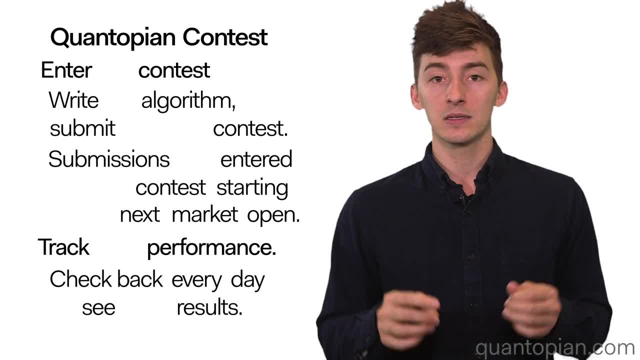 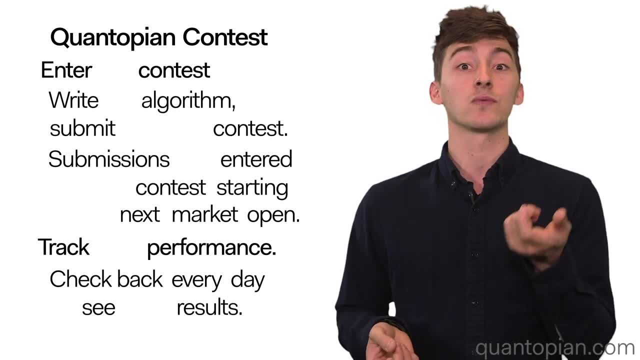 word in the corpus, but they take a different approach. Stemming takes all of our words and just chops the end off of them. It's a super crude heuristic, but it gives us this base root word that we can use, While lemmatization is a little bit smarter in how it actually goes about it. 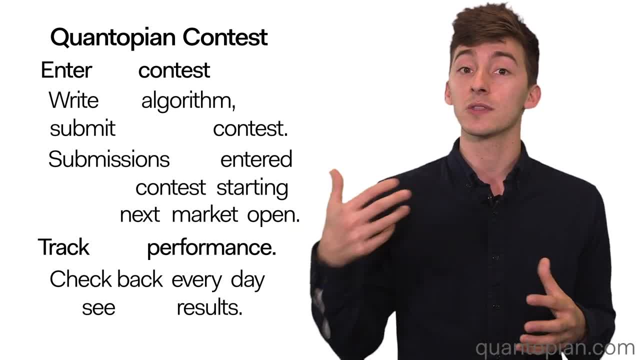 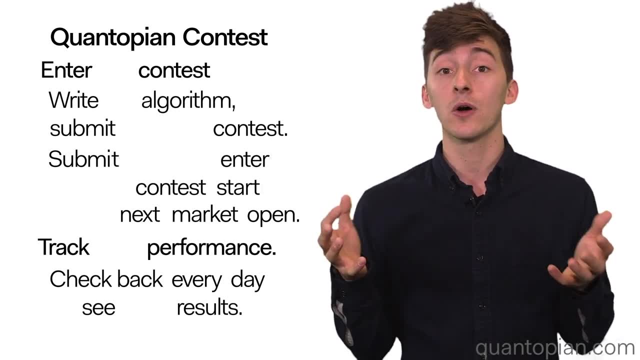 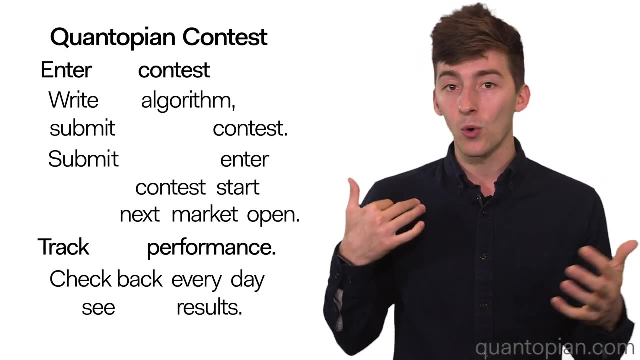 It actually uses a vocabulary and analyzes all the words in the corpus to get the actual root word. These are two different options that you can use basically to break down our tokens into the root individual words. We can normalize all of our text Now once we have our stemmed or lemmatized. 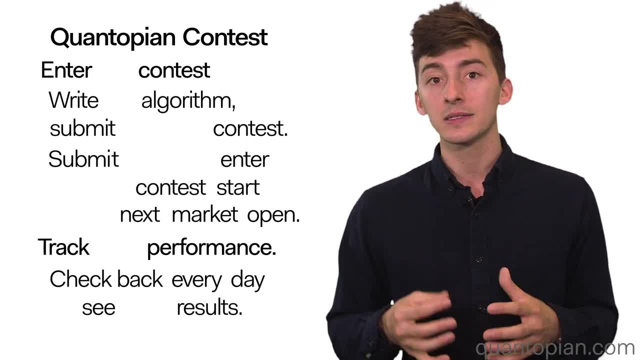 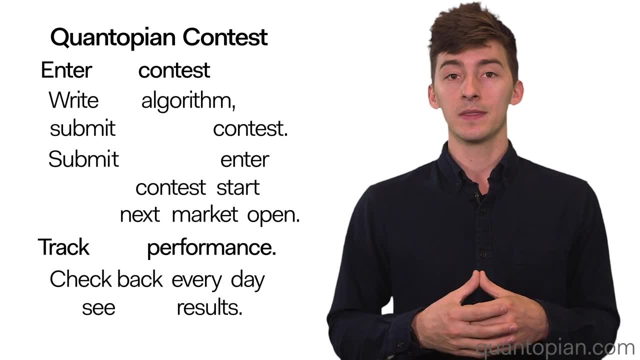 corpus, with all the stop words filtered out, with everything tokenized. we can actually try to quantify this, And the way that we can actually go about this is using a bag of words, And this is a pretty simple concept in natural language processing, used a lot in machine learning. 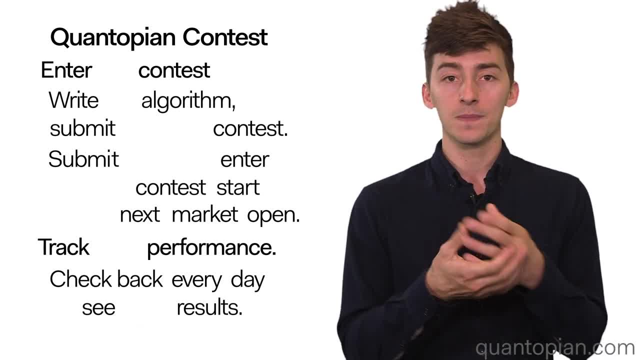 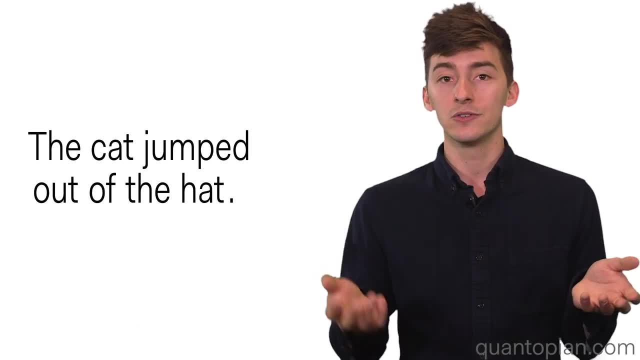 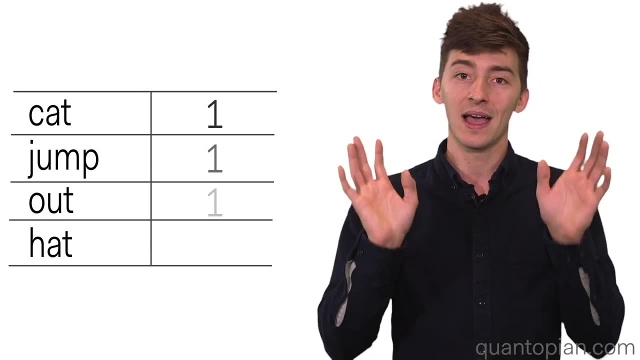 where you essentially count all instances of all the tokens in a given observation. So in some document there would be the cat jumped out of the hat right. All of those would be individual words and they each occur about once after removing the stuff like that. So the vector, 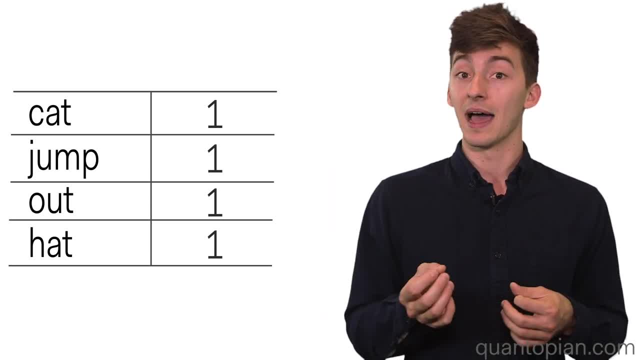 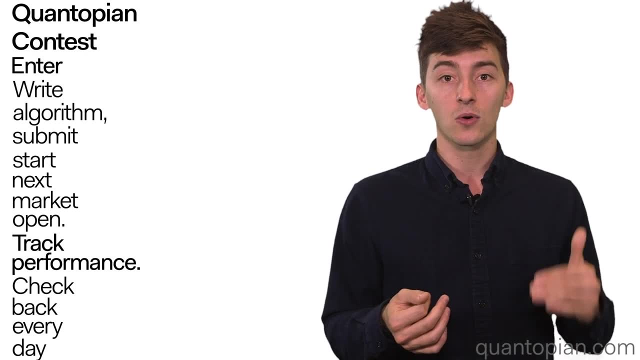 that represents that document would have like a bunch of ones and zeros For each of the one words that showed up in it. Basically, for every single document in this corpus, we count every single instance of every single individual word in it So that we eventually end. 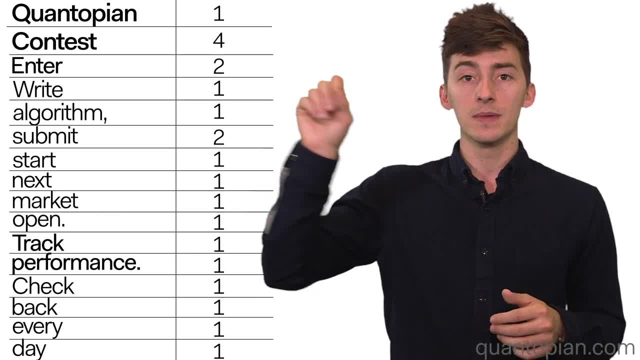 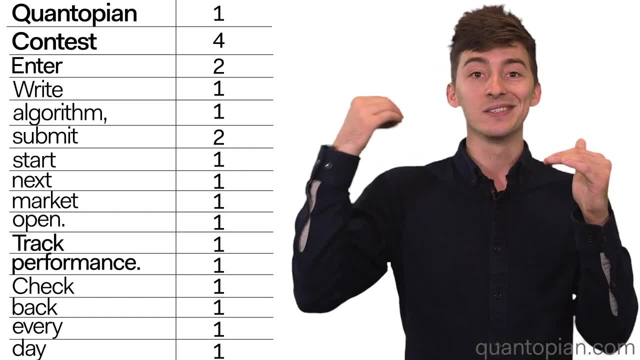 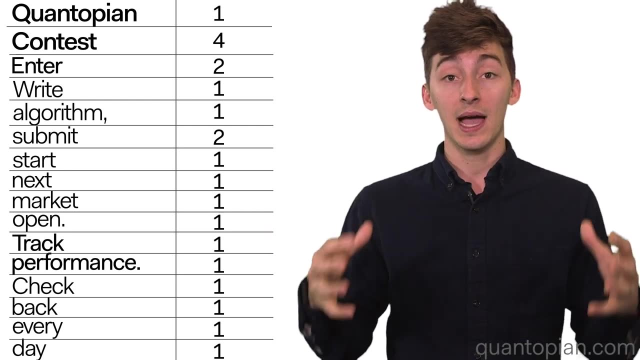 up with this big matrix where every single column is the relevant token, and then every single observation is the document, And then we have zeros or higher integer numbers for the number of times that a given word appears in that document. Once we have this, we can. 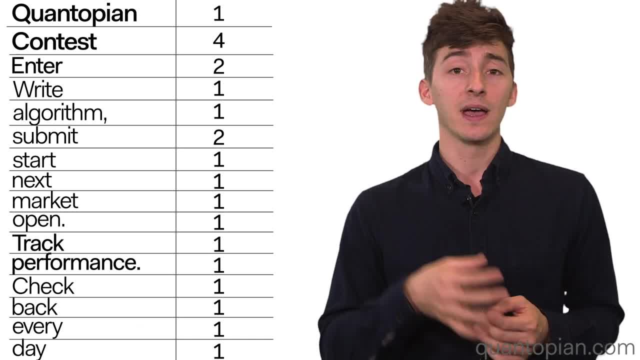 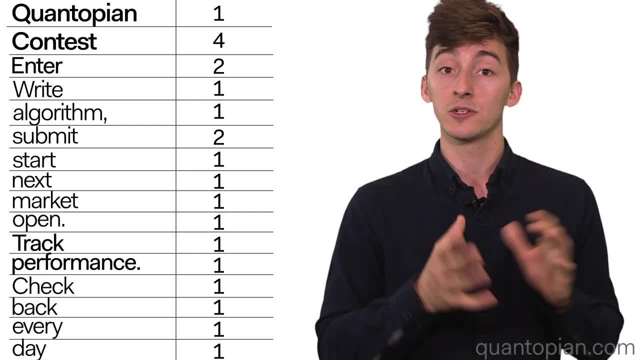 use this for whatever modeling purposes that we like. If we have labels such as positive or negative sentiment, well, we have the appropriate vectors for everything, So we can just build our sentiment model using our feature matrix. If we want to predict something else about these documents,